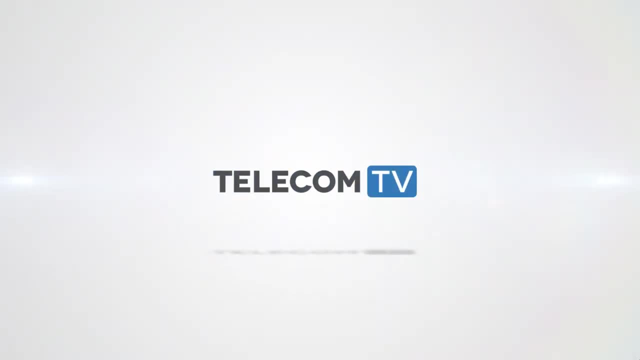 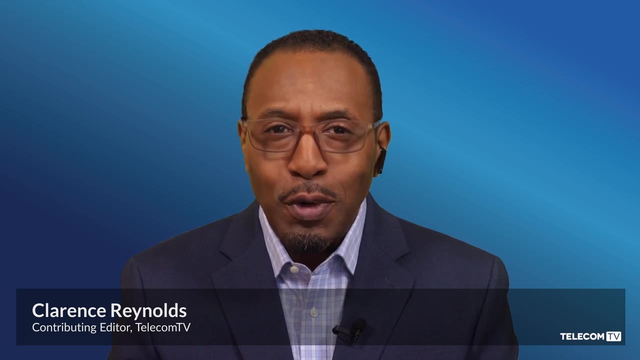 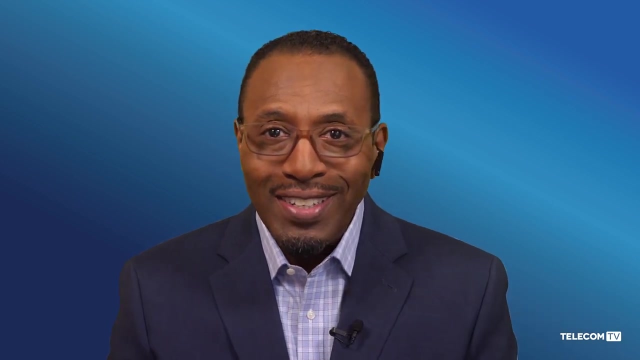 The telecom industry has long been on the verge of revolution, and this year's milestones reinforce that stance. So what have we learned and what new frontiers will we face in 2024?? Caroline Shan, VP of the Network and Edge Group at Intel, joins me with a look back. 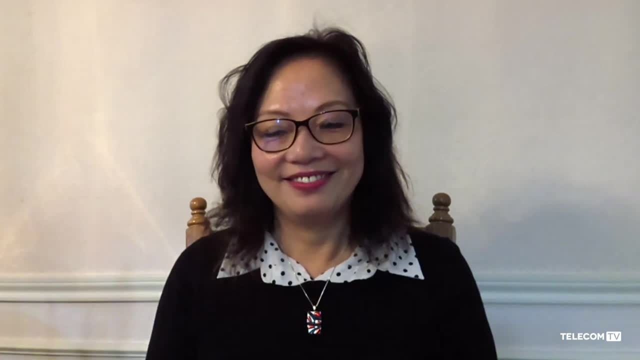 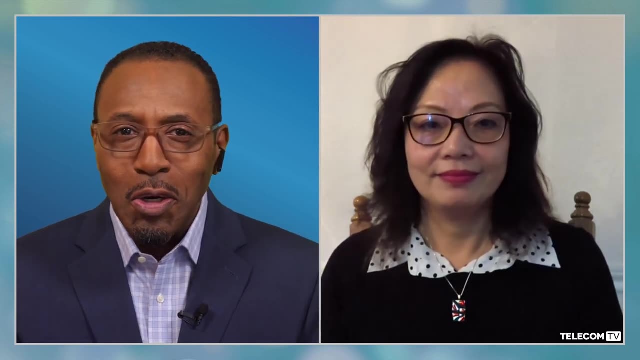 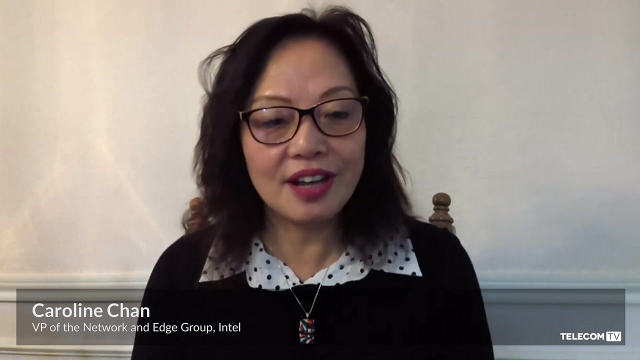 at the developments of 2023 and her outlook for the year ahead. Welcome, Caroline. So, as we wrap up 2023, any thoughts on the year and the current state of the telecom industry. So we are continuing to see the desegregation of hardware and software that is happening. 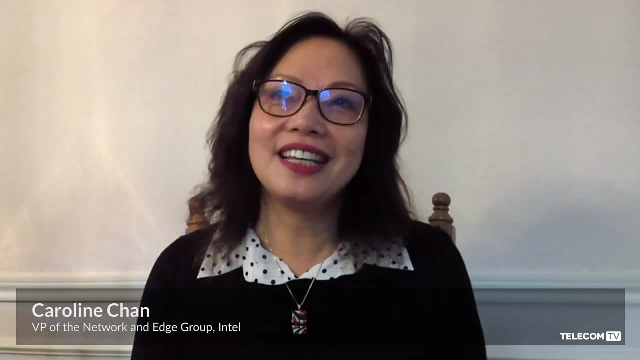 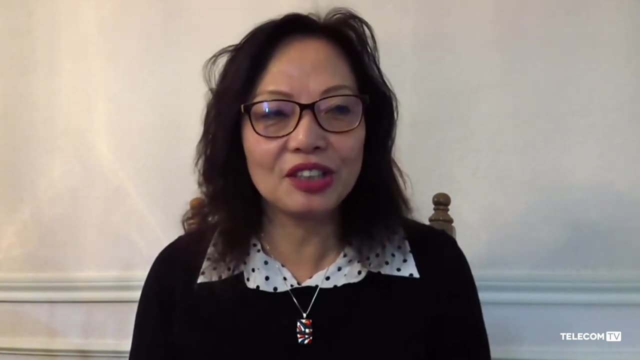 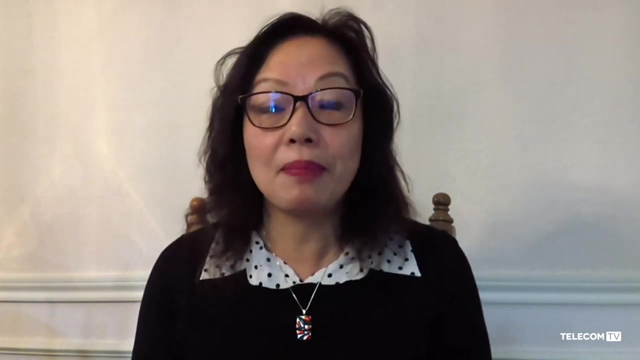 in a faster pace than ever. We see VRAM and ORAM gaining momentum, although still at a smaller scale of the total market, but the momentum is definitely there. I think the other key thing that really popping up is sustainability- power consumption That is not just something that's. 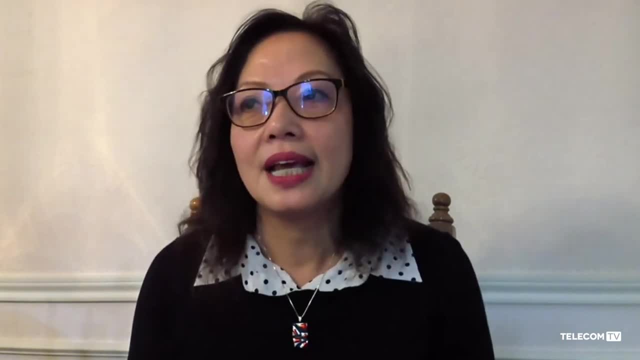 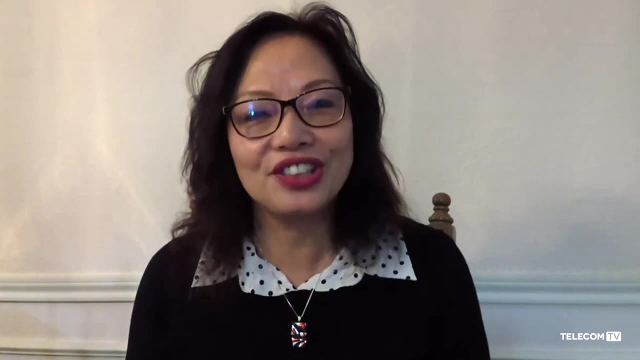 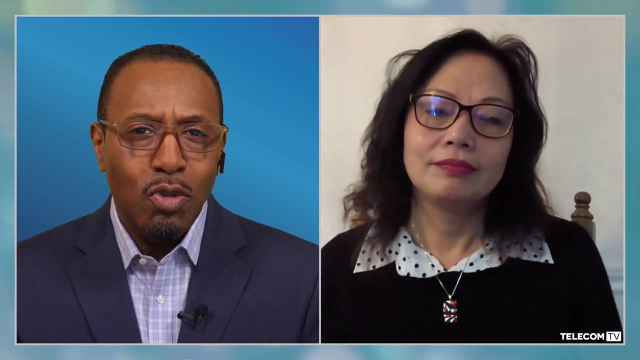 facing the telco industry, but facing all industries, And no one can deny the momentum of AI. AI is changing everything. It's definitely also changing the telecom industry, So it's been a very interesting year. Have you heard any recurring themes or priorities that come up? 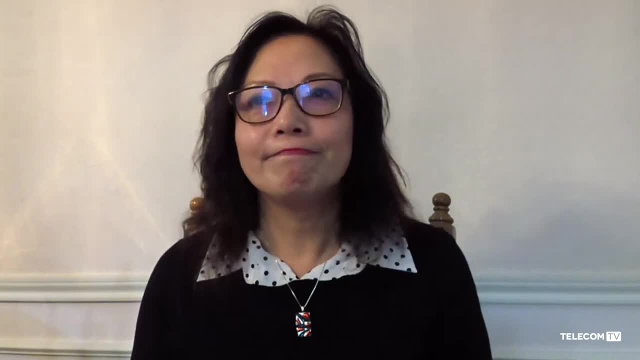 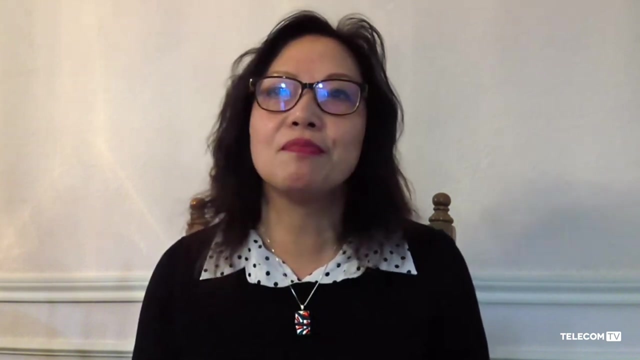 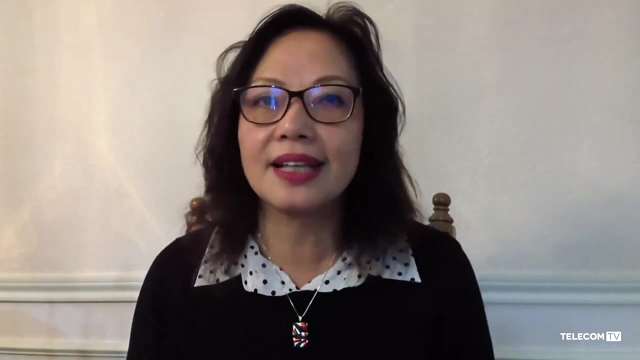 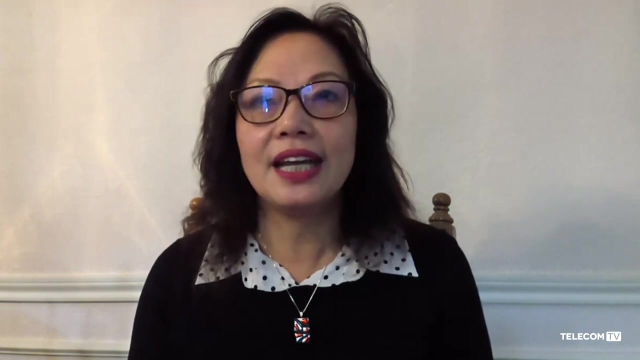 in your industry conversations- Sustainability. Many times it's an industry initiative, Sometimes it's also a government mandate. How do I get more out of the network that I deployed, In other words, return of investment beyond just the consumer side? So some things like edge H-A-I private networks, taking 5G into the enterprise. 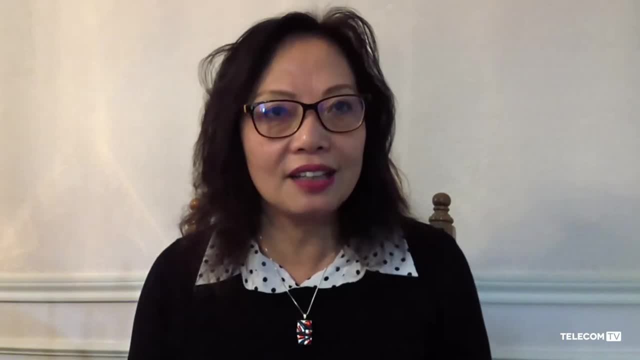 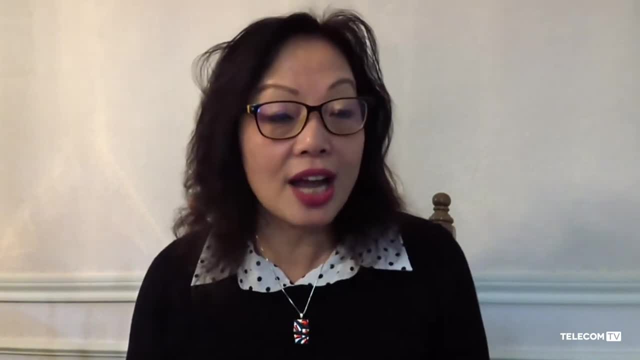 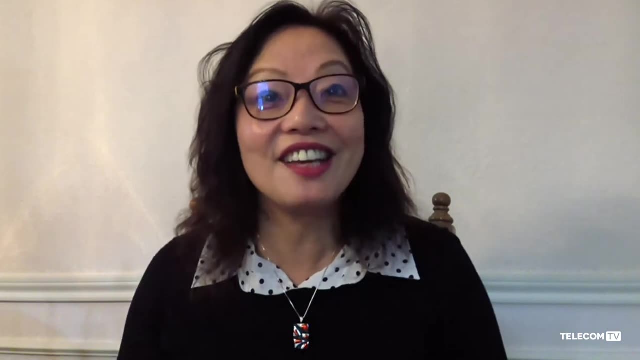 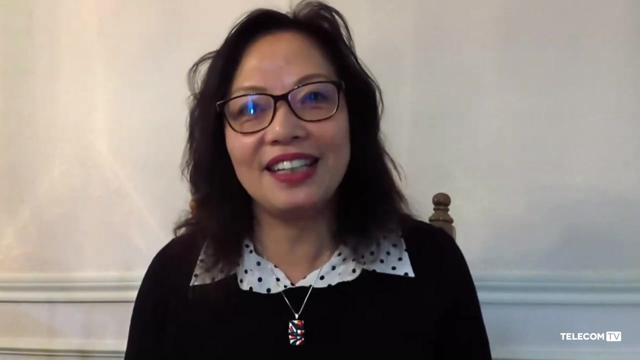 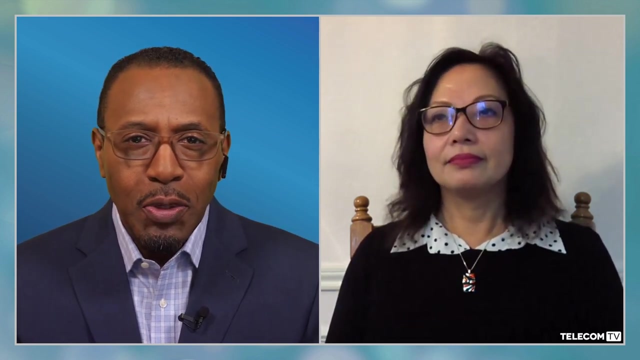 desegregation. it is posing organization challenges to many operators. So how do I make it such that I put the pieces back together effectively and efficiently at a total TCO, much lower TCO? That has been the recurring theme. So, Caroline, as we move into 2024, what's the greatest area of opportunity and